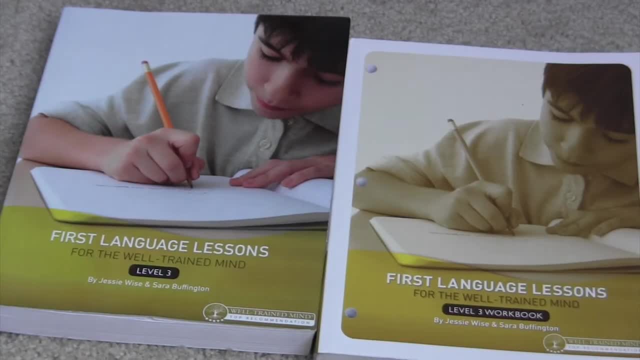 Hey guys and welcome back to my channel. Today I'm going to do a review of first language lessons for the well-trained mind, level three. This is an excellent curriculum for teaching grammar, writing, sentence diagramming using a dictionary, learning how to not just write in correct grammar. 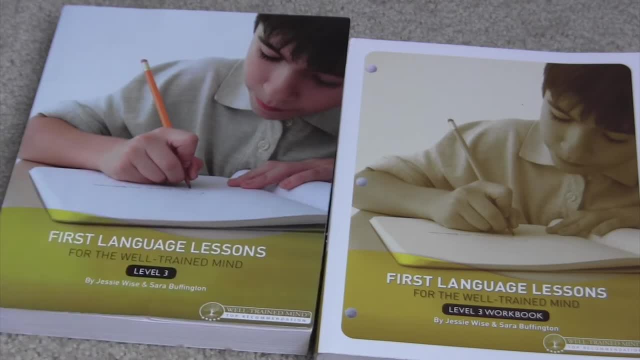 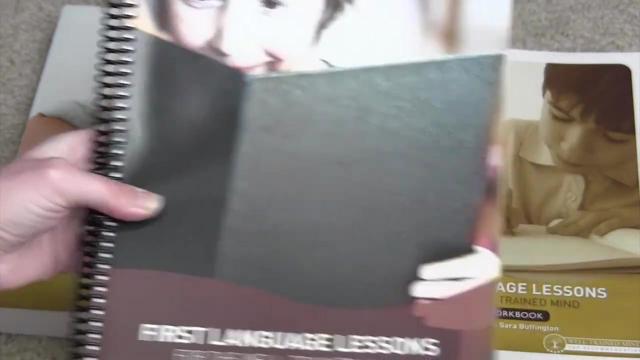 but speaking in correct grammar, and I'm just going to talk to you a little bit about it today. Now, if you see my other reviews, I reviewed level one. I can link that below. I also just finished filming first language lessons for the well-trained mind. level two: I will link that. 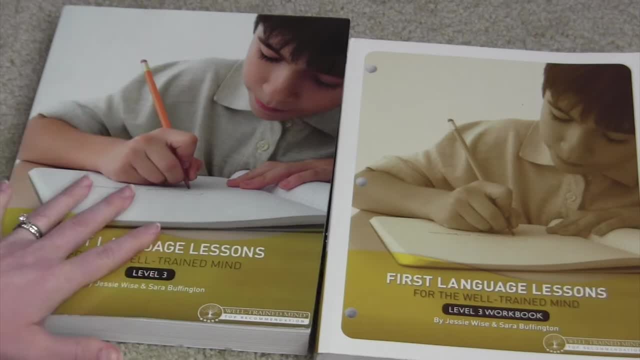 below as well, but this is an excellent, excellent, open and go language arts curriculum. I am doing this currently for my oldest son, who is in fourth grade. We did level one when he was in second grade, level two when he was in third grade. 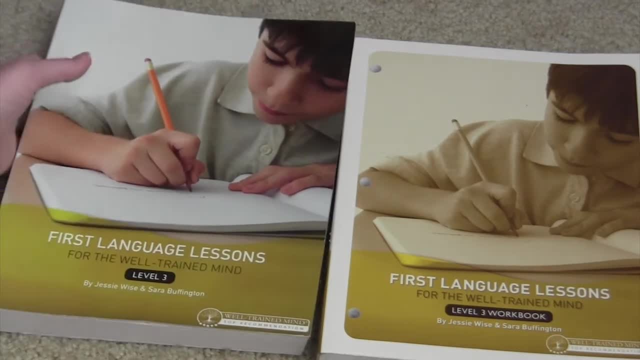 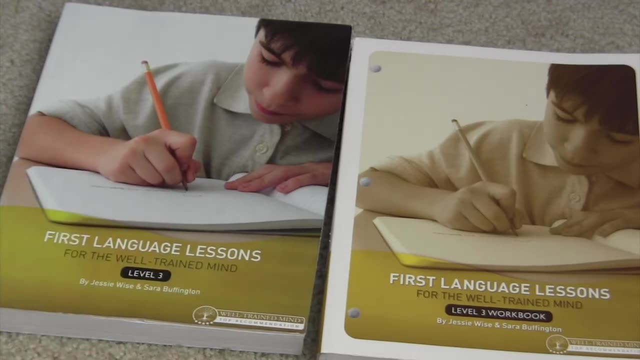 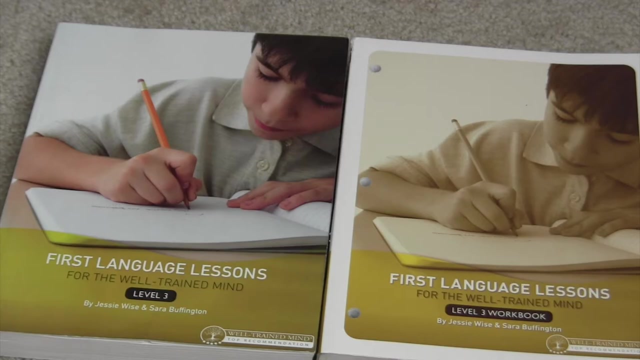 And we are almost finished. Like I think, we have five lessons or so left in level three and he's going to be in fifth grade in the fall. Time's going too fast. But we loved the first and second levels so I thought why not jump into the third? And this is the teacher's guide. It is not. 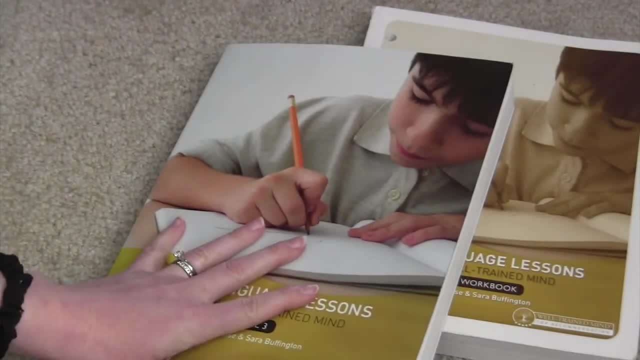 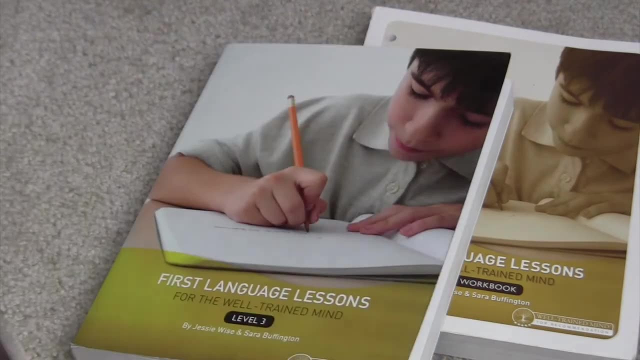 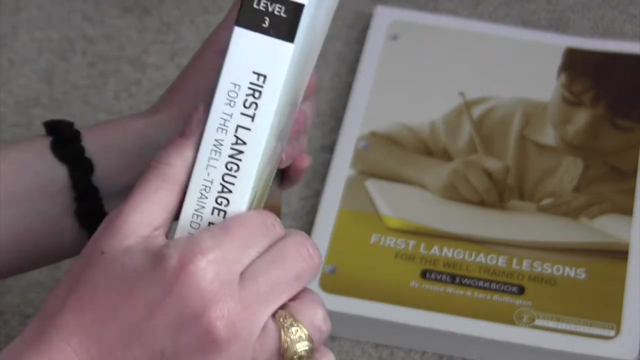 consumable, so it's something you can use for multiple children. if you decide to use this for multiple children With my level one and two, I decided to get it coil bound. But because this is so huge, it's so thick, so much thicker, I decided if I coiled it it might not hold its structure on my bookshelf. 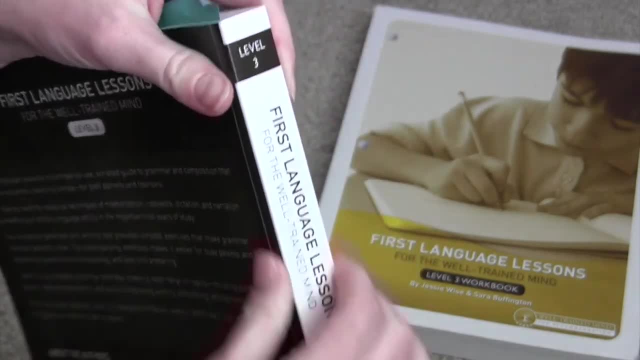 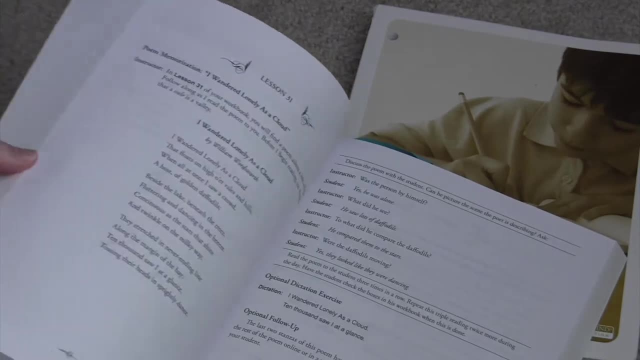 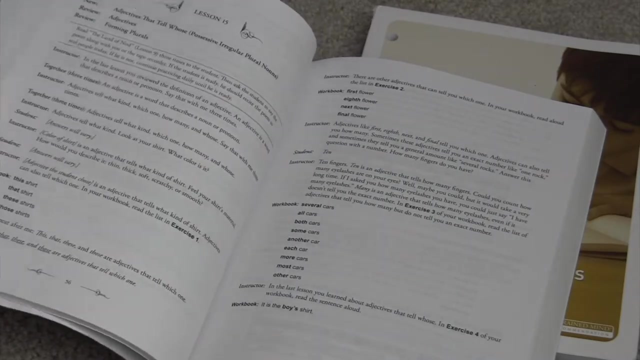 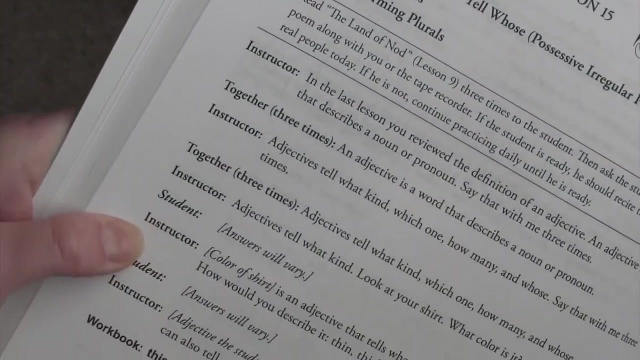 and may not live as long because this spine is super, super, super strong. So I decided to leave it like this. But this is the teacher's guide right here and it looks very similar, just black and white, Very similar to lessons to levels one and two And, just like levels one and two, it is scripted. 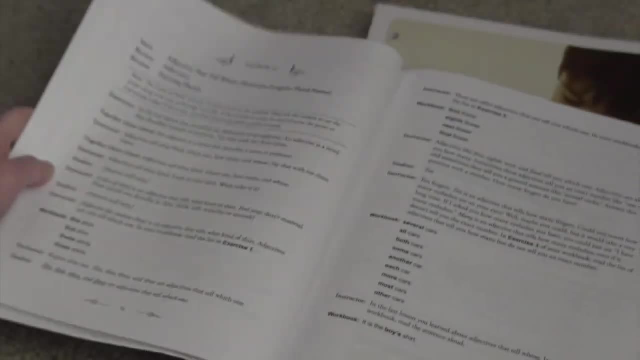 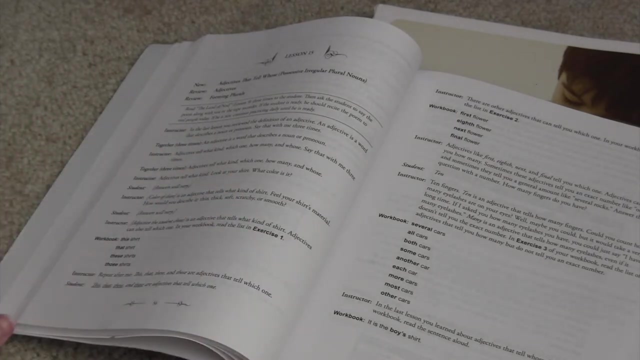 What a beautiful thing. This is very much open and go. I don't prepare, if we're being honest, I don't prepare at all for this. Sometimes you do a lesson and it'll say at the end of the lesson: hey, just. 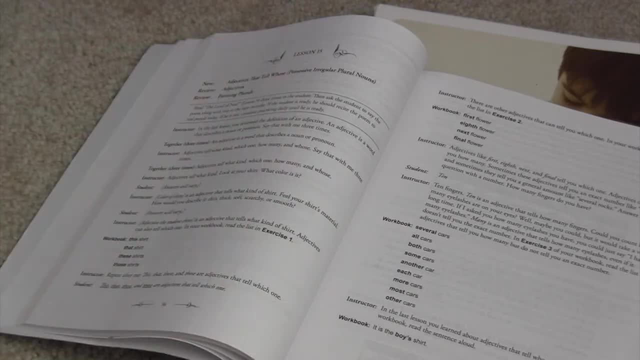 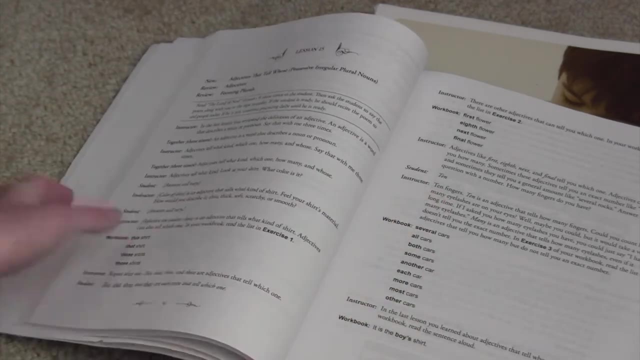 so you know we're going to learn how to write names and addresses next time. so make sure you've got some patience, Or make sure you've got a chalkboard or a marker board or whatever. But this doesn't require anything else except the student book, which I will go into in just a minute. But again, this makes 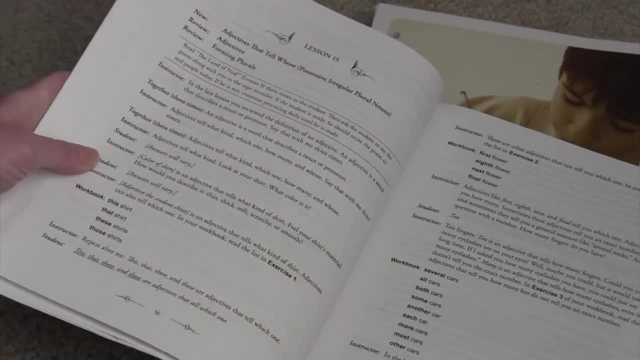 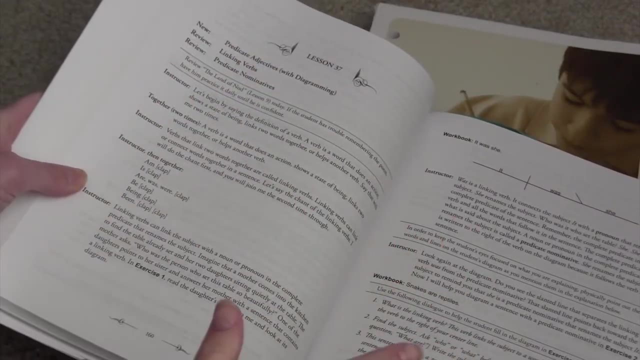 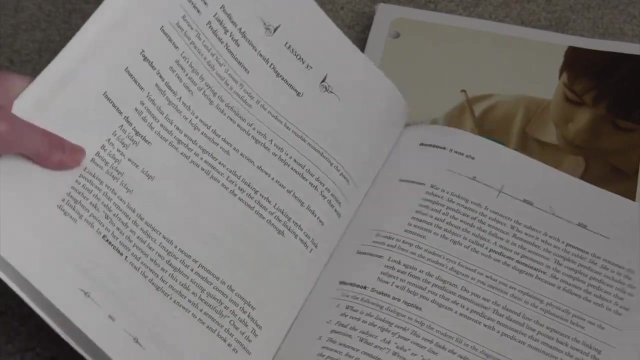 teaching grammar, writing poems, all of that. it makes this so easy. Diagramming sentences: If you don't remember anything from school about diagramming sentences, no worries, because it's all here. This will refresh your memory and it's complete. 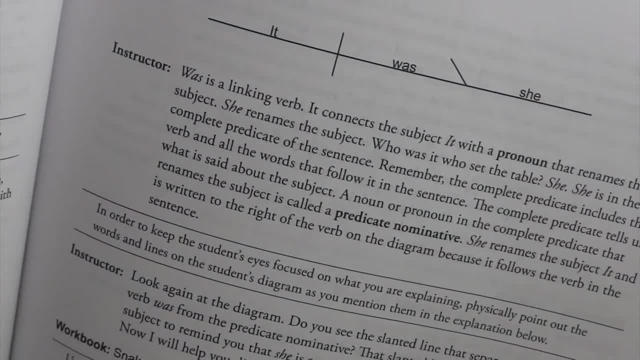 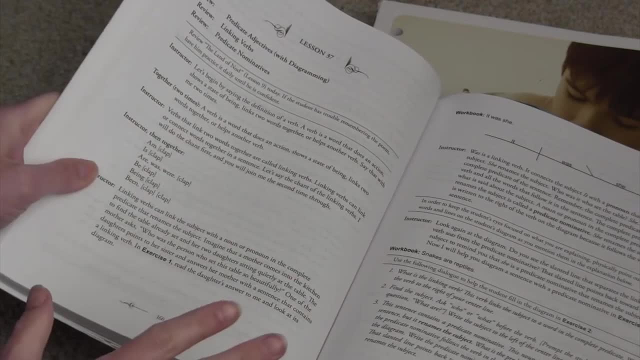 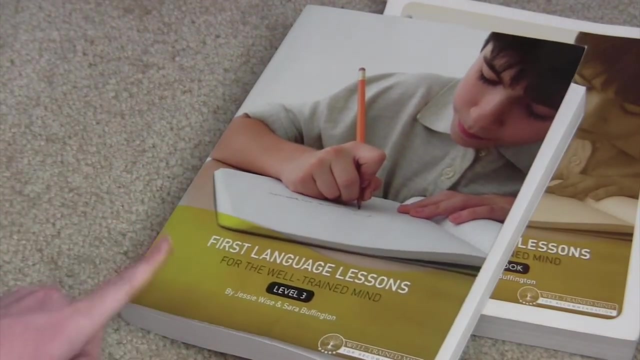 And totally scripted. Isn't that beautiful. I have learned a ton, I've been refreshed a lot with this And I think that this is absolutely fabulous. Next year, my oldest is going to be in IEW Institute for Excellence in Writing And I believe that this has given him an excellent foundation for next. 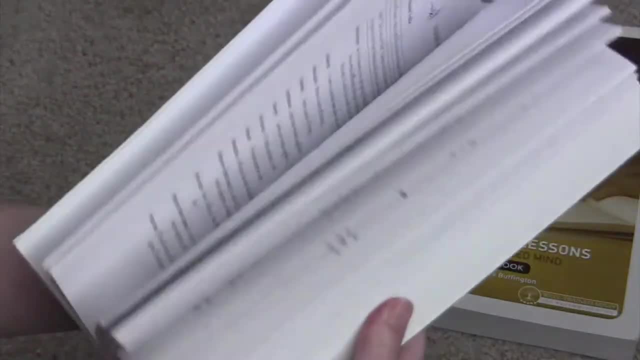 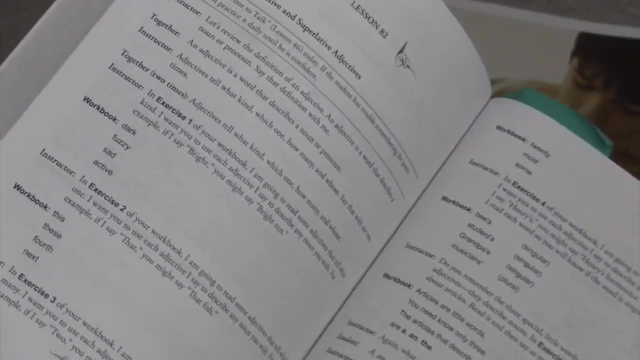 year, when he'll be in fifth grade. So, like I said, this is the Non-Consumable Teacher's Guide. I know it's boring y'all, but the content is so good. Meaning: boring: meaning black and white, no pictures. 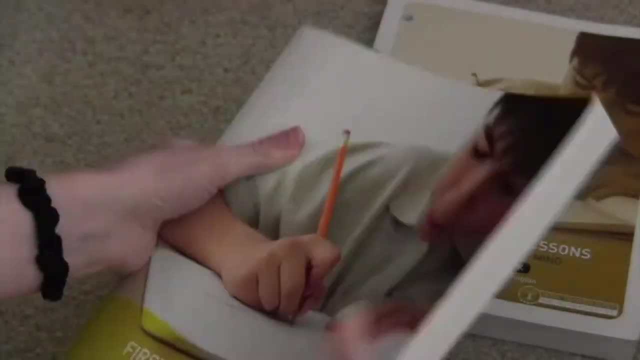 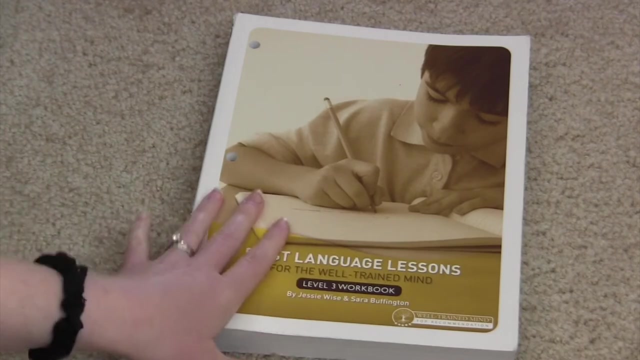 But it doesn't matter, It is just so good and tells you exactly what to say. Now the student book is consumable, 100% consumable. You will not be able to use this from one student to the next. It comes. 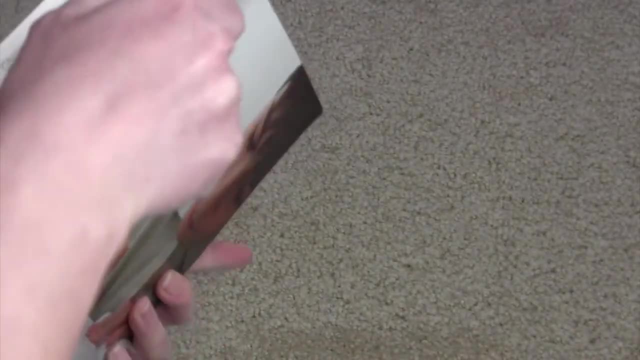 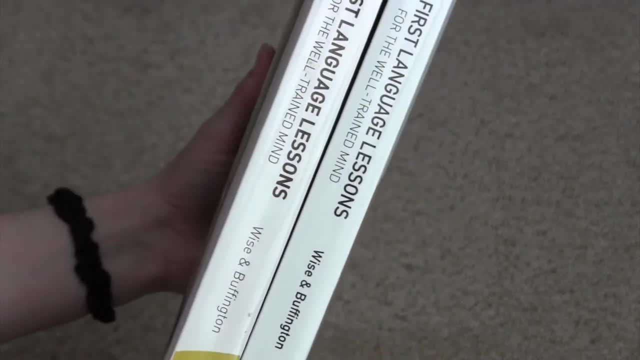 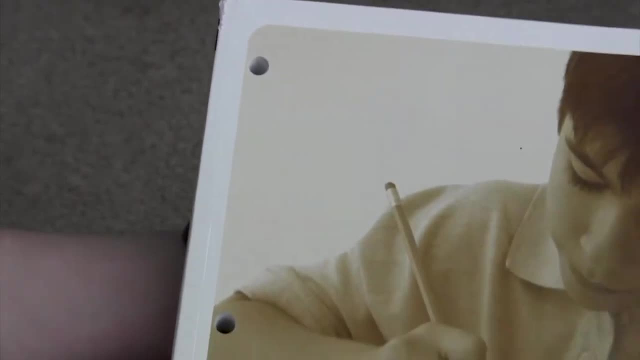 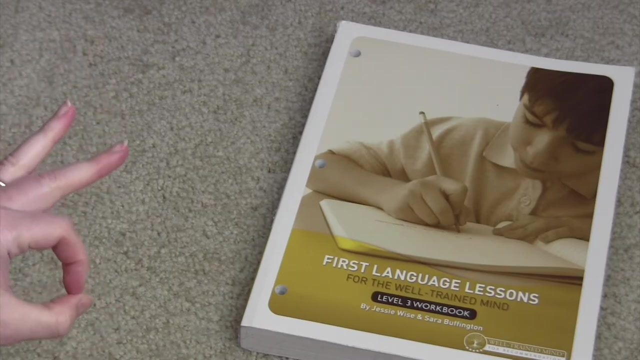 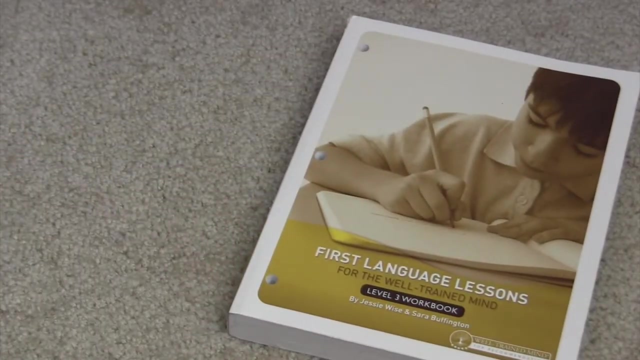 size, But this one comes hole punched and I have seen this put into a binder, but I just decided to keep it as is. I am personally a lefty and so if I were the student, this would have driven me absolutely crazy, But I have a right-handed fourth grader, so I just kept it as it was. But as 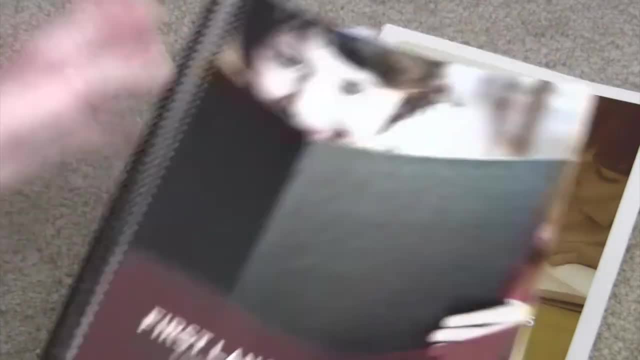 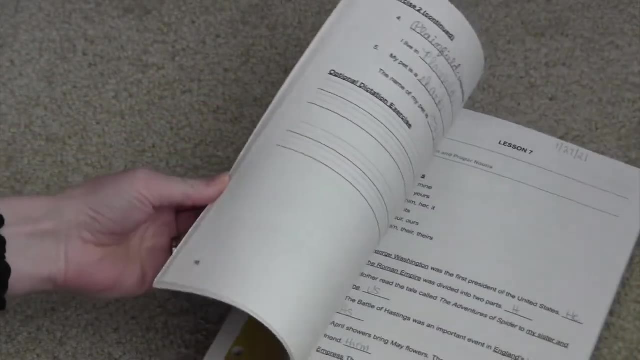 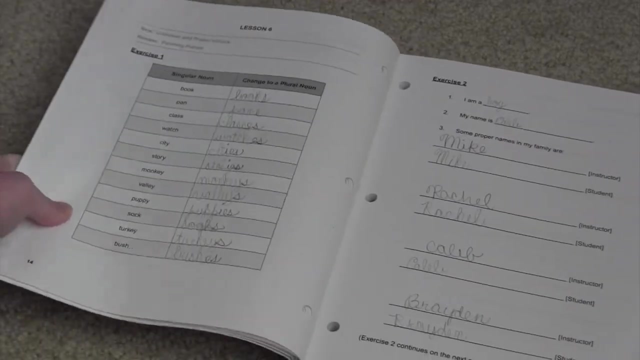 opposed to levels one and two, which are like this. you don't need a student book. this, this is a must-have. you cannot do it without this. so this book, it's, it's everything. it's um, let me see if I can zoom in a. 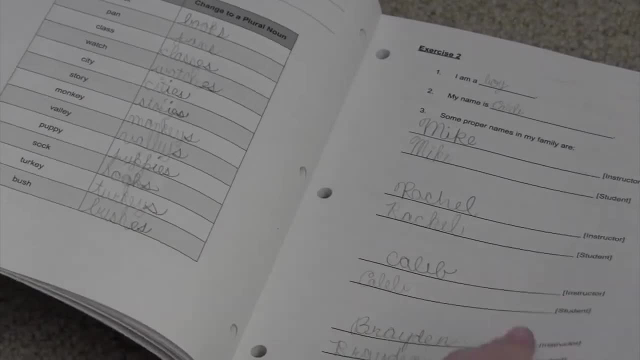 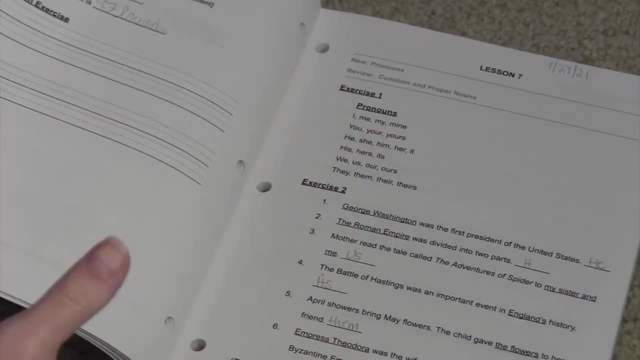 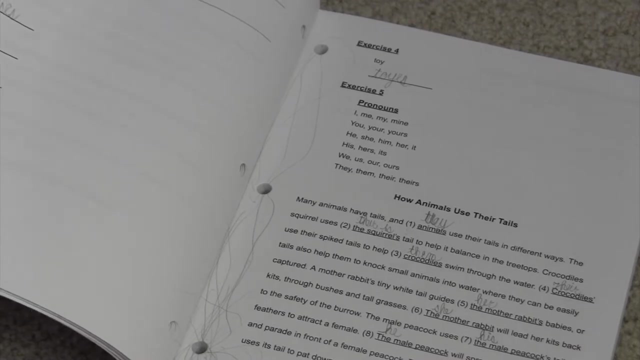 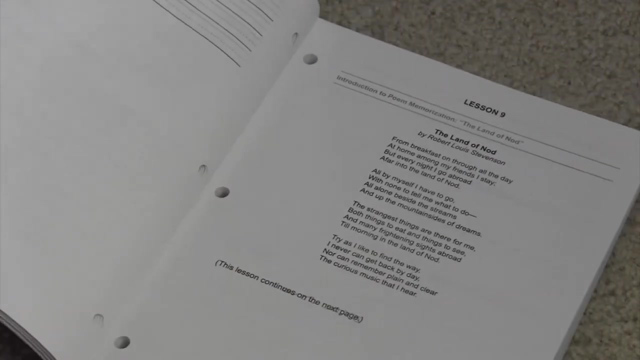 little bit. we learned about proper nouns, common nouns, pronouns, going over everything that we learned in lesson levels one and two. we learned how to pick out different parts of speech in and you know a paragraph or so. there is a lot of poetry memorization in here and we actually kind of enjoy these poems. 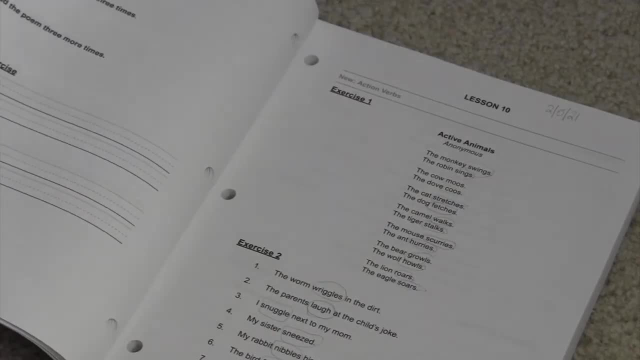 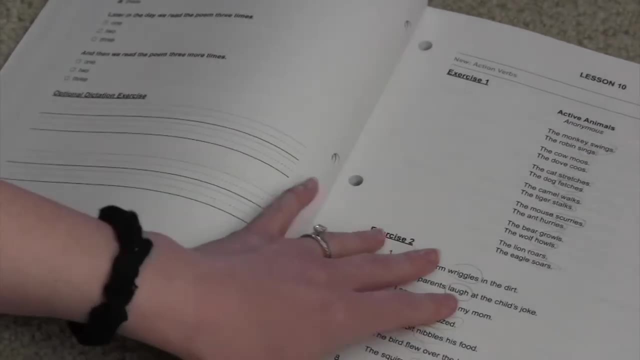 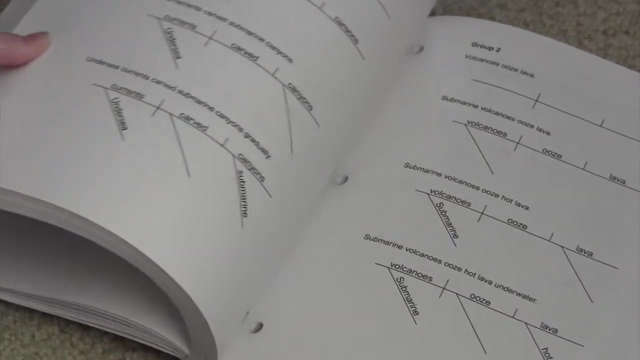 okay, I enjoyed the poem. I have a boy. they're not so much into poems sometimes, but yeah, and so picking out different things that they've learned, basically tuning in and out of the book, is a great way for us to learn more about the their eye to see different things in order to diagram sentences. so this is 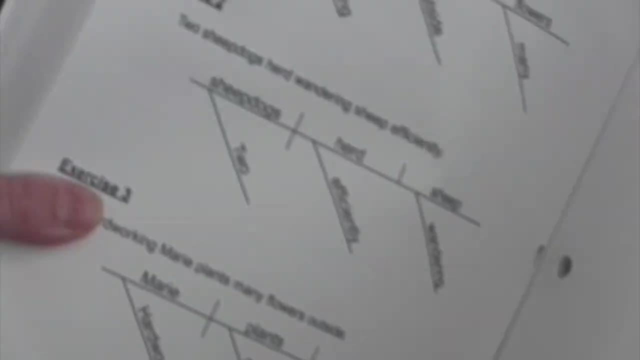 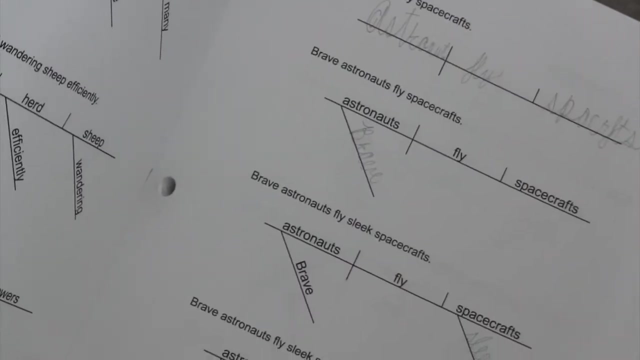 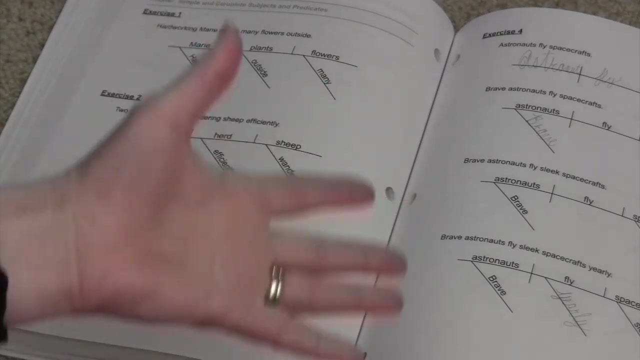 just one thing. okay, this is lesson 60. it shows how to do them. and then here he is doing it there. now this looks like: what do I do you, you, you, you may look at this that they go. can I just get this book and not the teacher's guide? 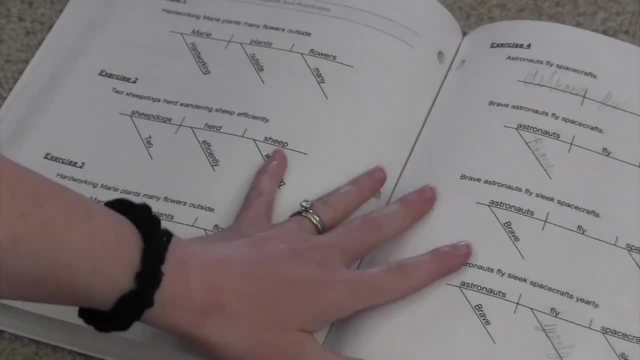 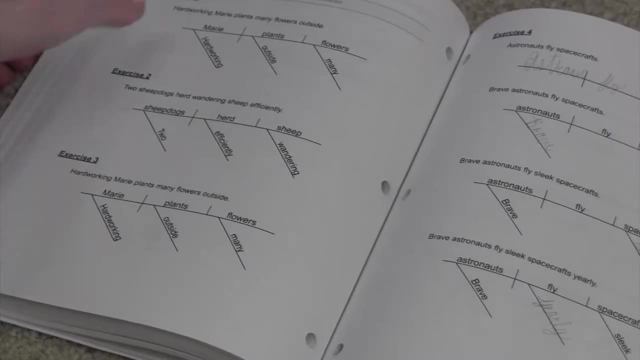 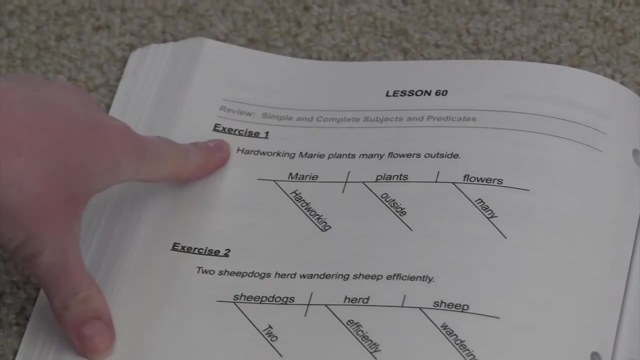 absolutely not. okay, this is lesson 60. let me open to lesson 60 in the teacher's guide. okay, I'm gonna read it to you here, just to give you an idea, and here's what he is looking at. okay, exercise one. let's see, I'll say every. 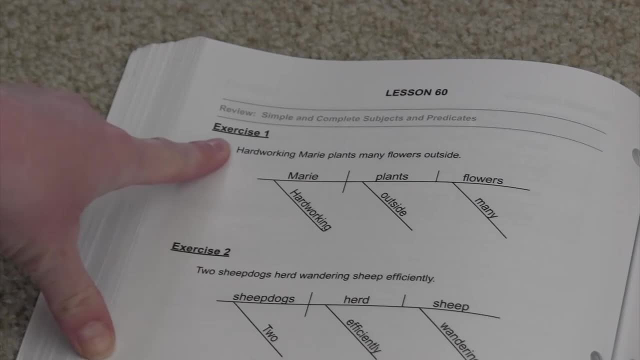 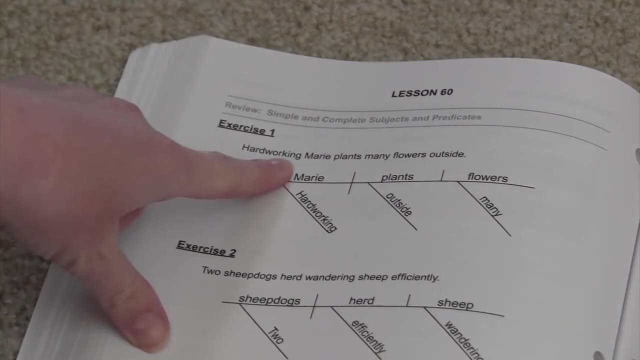 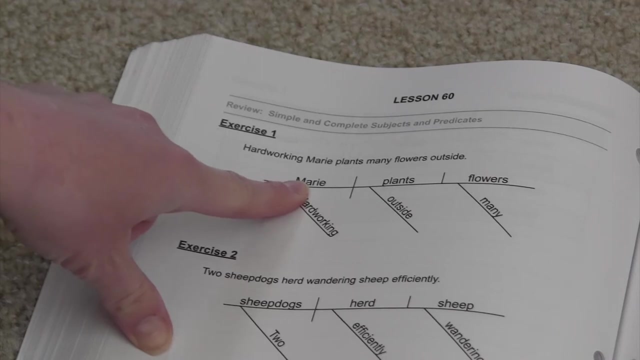 sentence has a subject and a verb. on a diagram, the subject and verb are separated by a straight line that runs down through the horizontal line. to the left of this straight line, you will find all the words that tell you more about the subject: Marie. the subject of the sentence is simply the word Marie, so it. 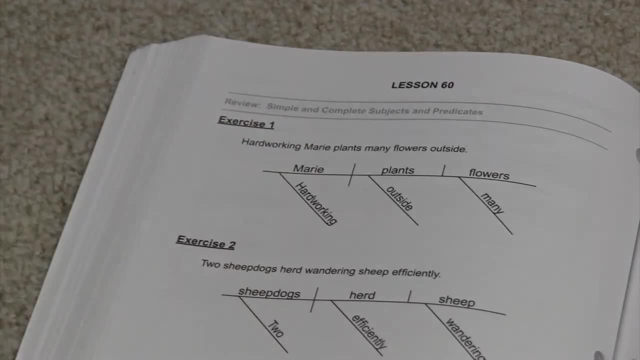 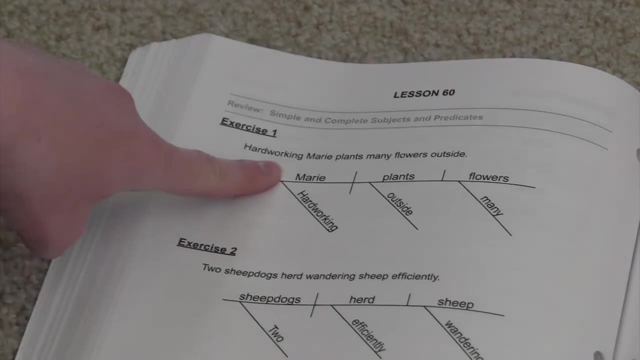 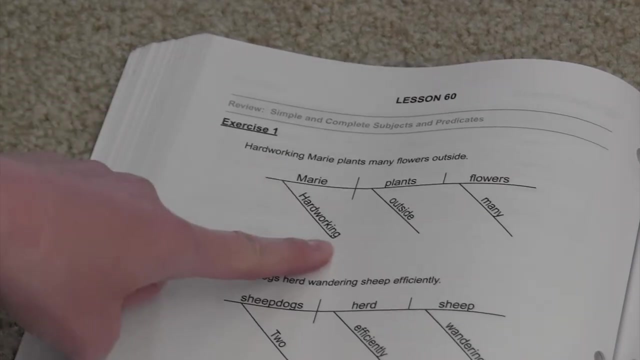 is called the simple subject. so it shows you. it shows you how to do all of these things. it says: look at the diagram and exercise one. the simple subject is always written on the subject line Marie. the complete subject is a simple subject: Marie. and all the words that hang off of the simple subject: hard-working Marie. 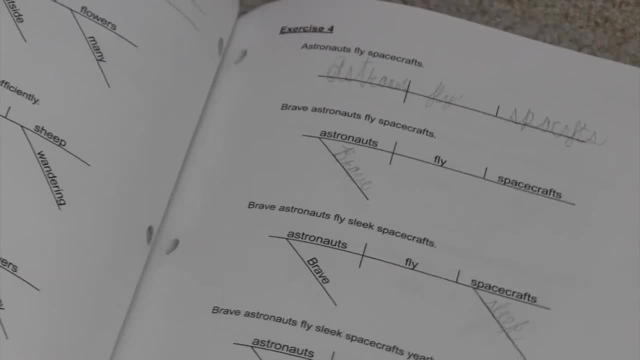 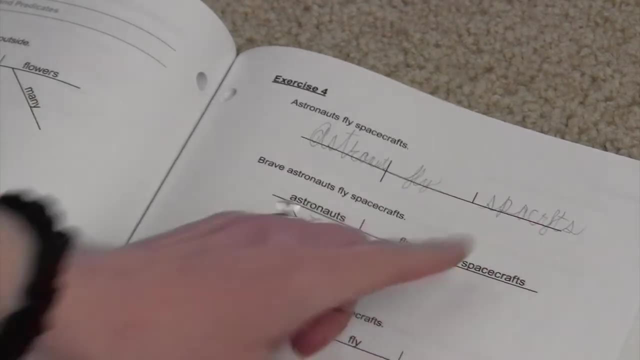 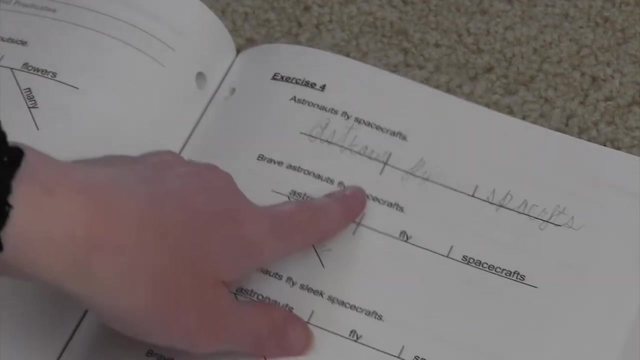 so yeah, and then when they start diagramming themselves, it gives you a bunch of questions to ask them. to walk them through it. like astronauts fly spacecrafts, what is the verb? I would ask what is the verb? and he would say fly. I say right, right, fly to the right of the straight line, so in the middle. so they 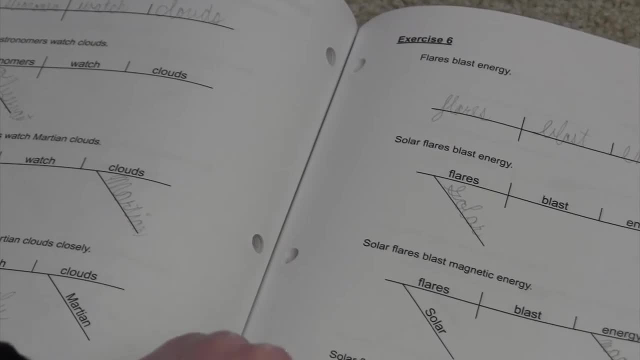 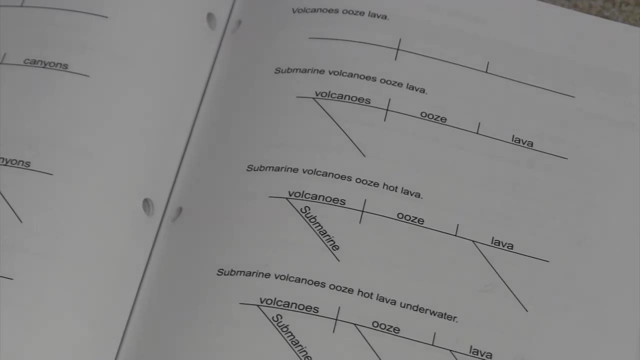 get over. you know, there's a lot of practice here and they get used to where the verb goes, where the subject goes, where the adjectives, the adverbs, the interjections that you know. all of that we learn about. they understood you and everything. so here's where we. 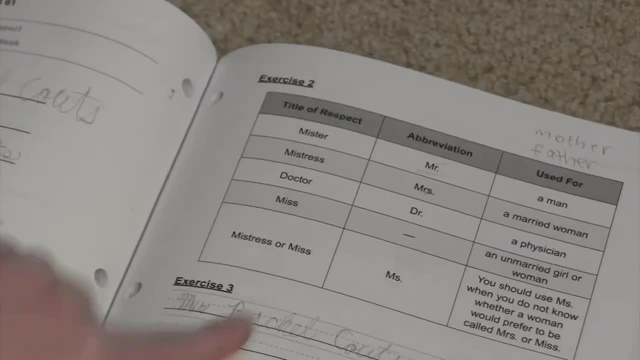 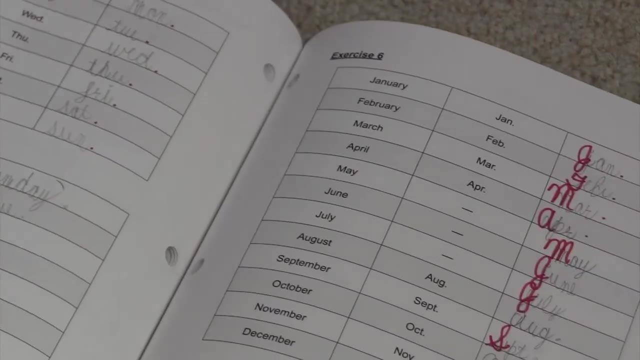 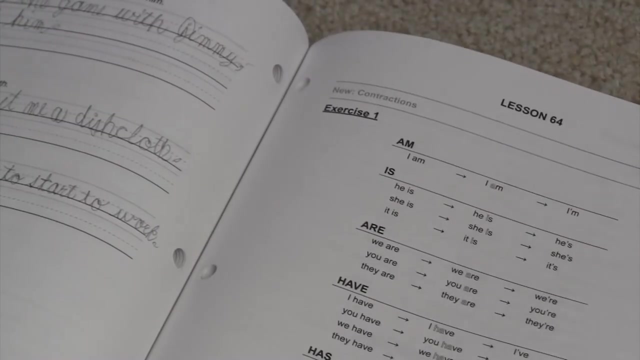 learned how to write people's full names. we learned about different titles of respect. we learned about days of the week, months of the year, how to abbreviate them. we learned about contractions. we learned about uh- where to put commas. here's some contractions like: he is becomes he is he's, she is becomes she's. 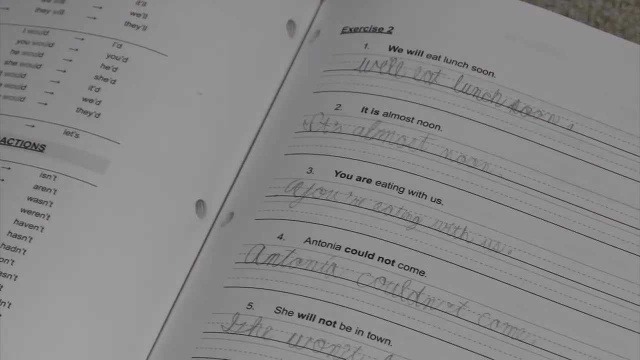 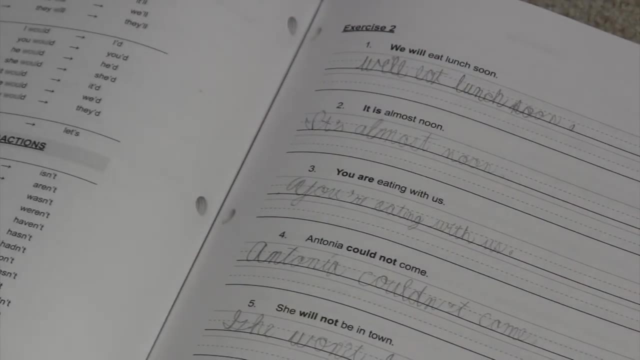 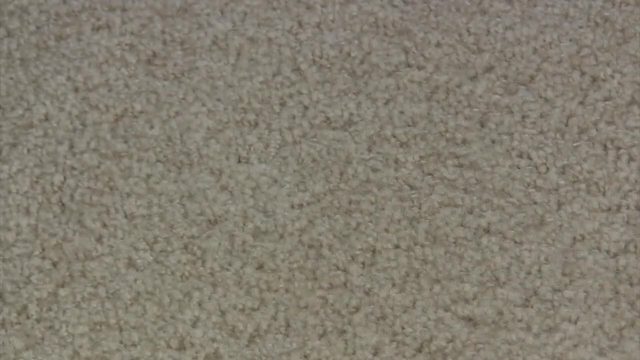 and that kind of thing. so yeah, but you can't just sit down with this and know what to do. you have to have the teacher's guide to walk you through it. so i hope that that is helpful. um, that's just the the basic stuff. let me back up a little bit. 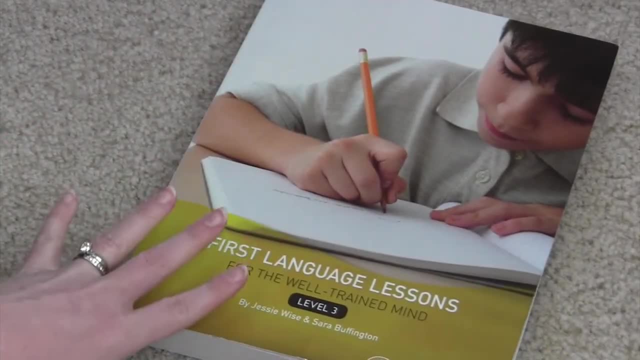 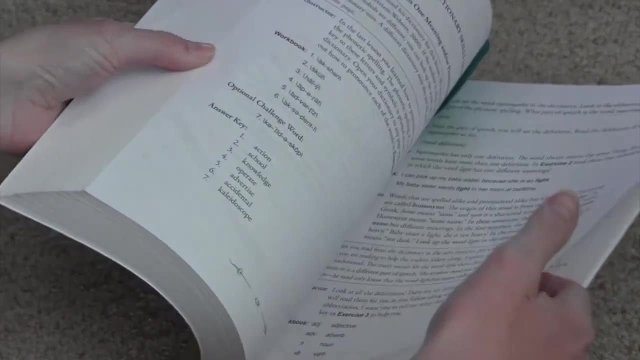 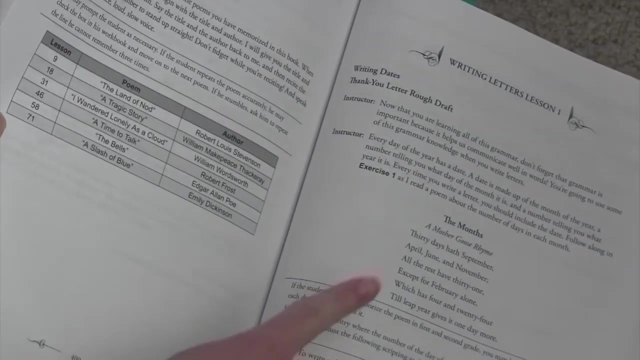 i thought when i jumped into this that this was all just diagramming sentences and poetry and stuff. but once you get to the back, let's see there are- okay, there are 89 regular lessons, and then there are writing letters lessons. so, uh, we learned how to do, how to write a letter. 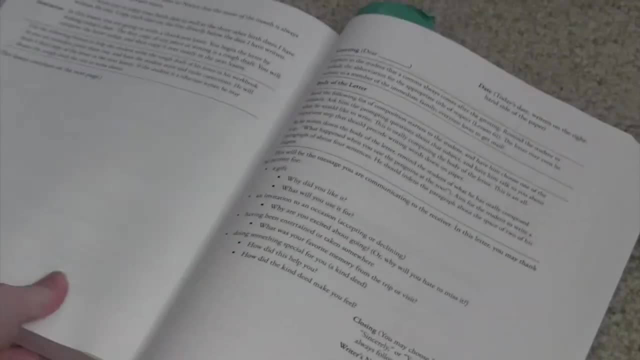 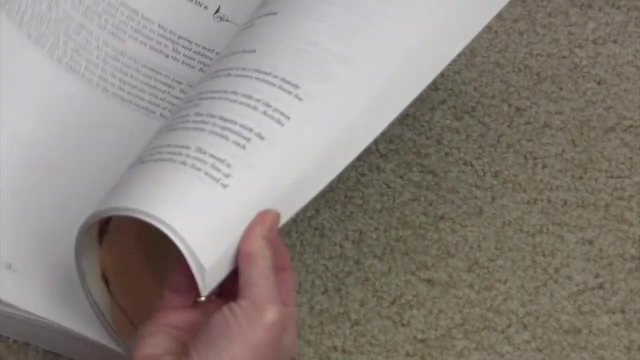 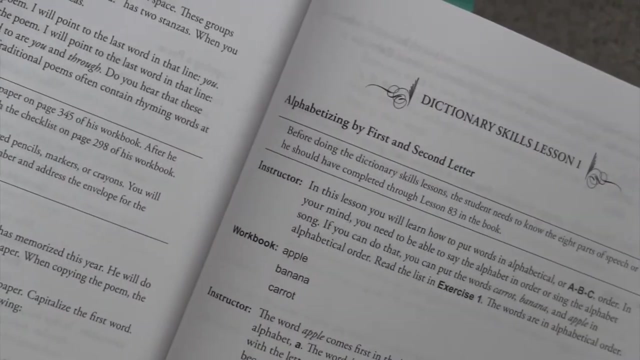 the proper way. we learned how to do a rough draft, final draft, and let's see, i can't remember how many letters. we learned how to write a letter and then we learned how to do a rough draft. there were, okay, there were seven letter writing lessons, and then there are seven dictionary skills lessons. 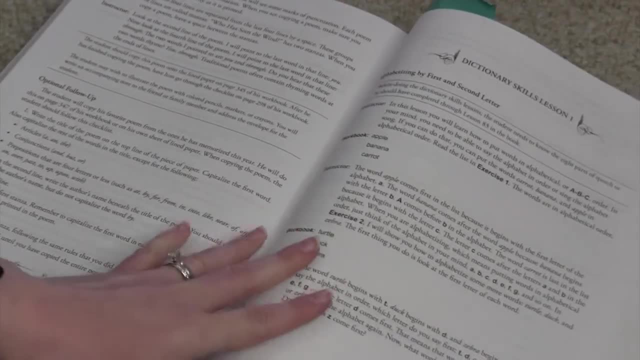 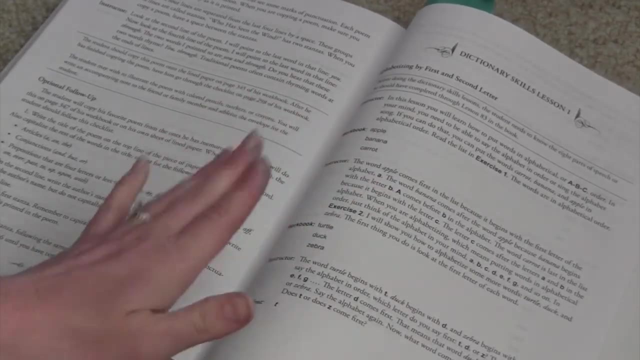 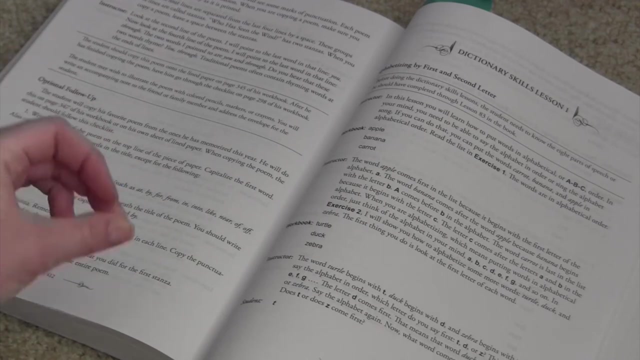 and this is seven lessons on how to use a dictionary, and this is what we're currently in. we did lesson five dictionary lesson five today and this is perfect. it teaches them how to use a dictionary and how to read the pronunciation, what the little symbols mean. we learned about syllables. 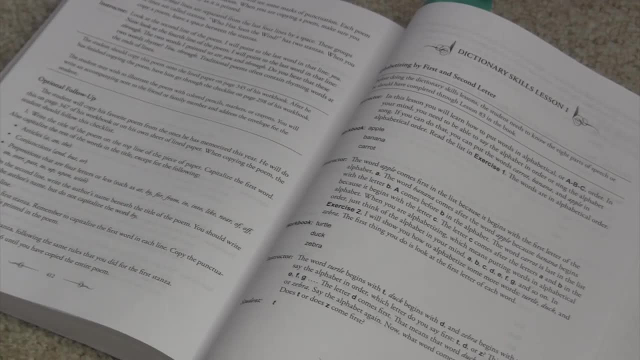 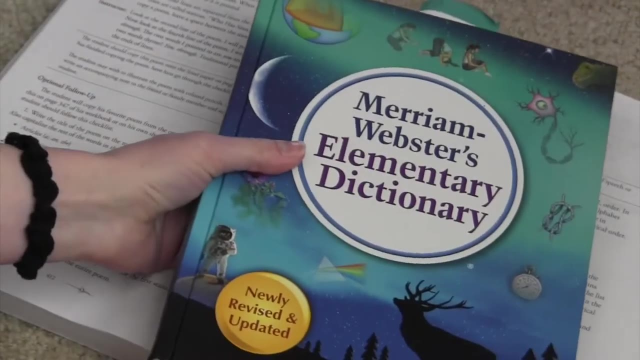 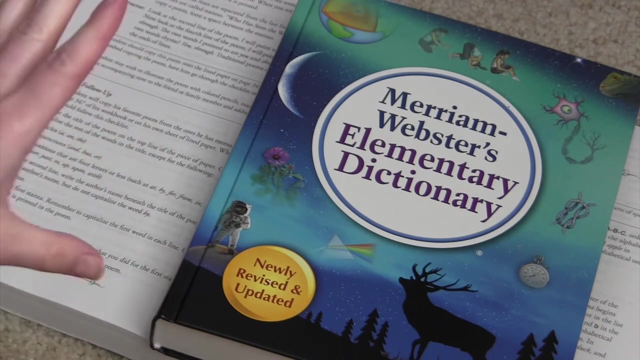 accenting on certain syllables, and the only thing that i've bought outside of the teacher's guide and the student book is this: this is the merriam-webster's elementary dictionary. it was recommended for this. there are several that are recommended, and this is so nice y'all like i wish. 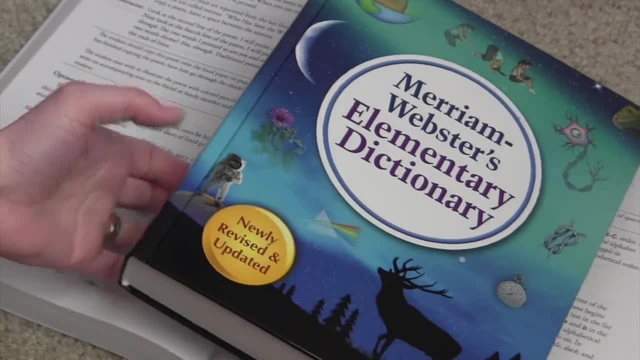 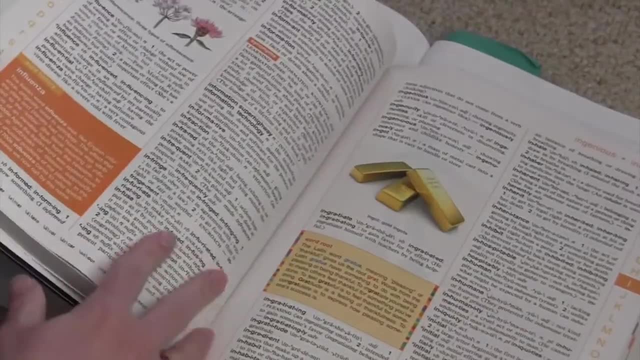 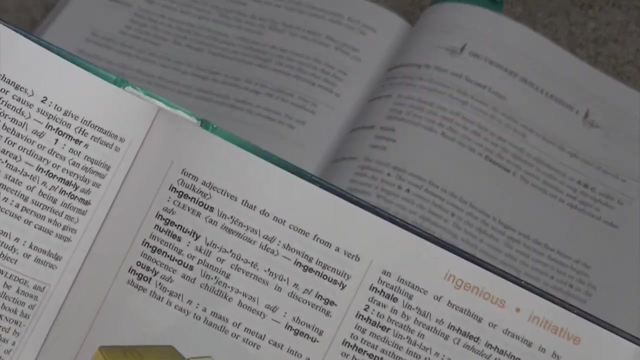 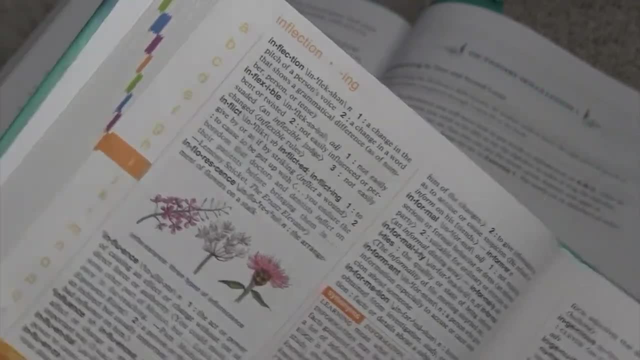 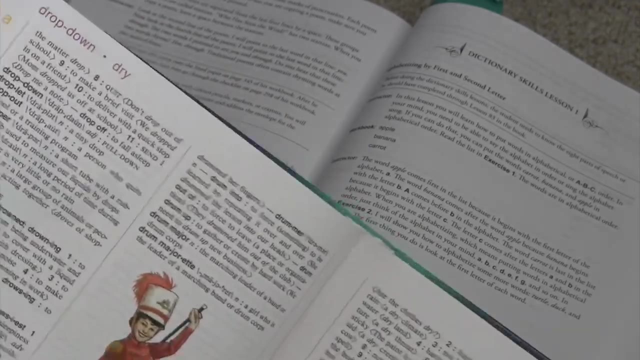 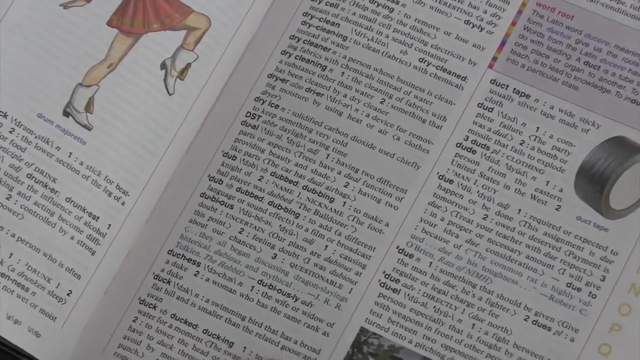 big print. you can see there. maybe i'll choose a different color so you can see it better. where's the purple? so nice pictures, big print, and this has been really good. and i told him. i said i don't care how old you are, you will for for. 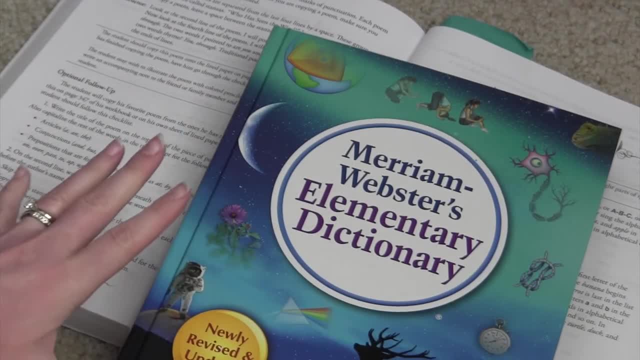 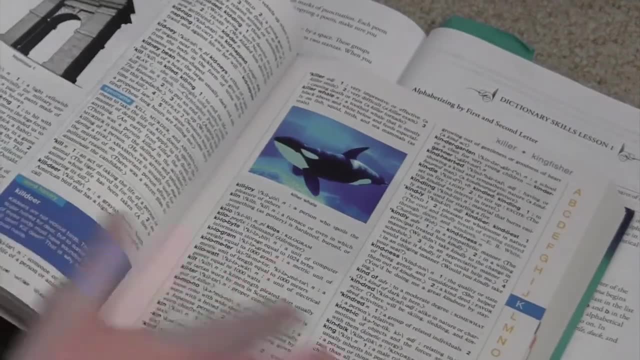 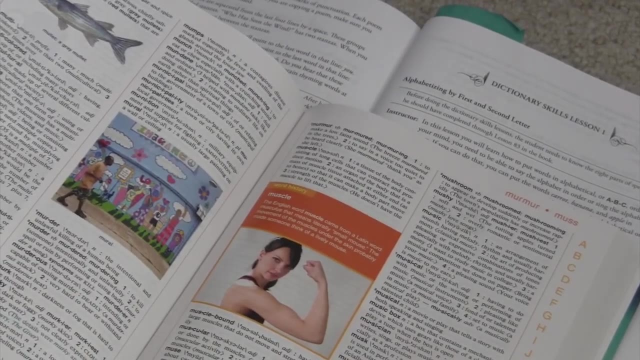 forever. when you're alphabetizing anything. you will still sing the abc song for the rest of your life. it never ends, and so we've just been learning how to find, how, to just kind of learn how to use these guide words to find the the right word that you're looking for, and i've really enjoyed this so. 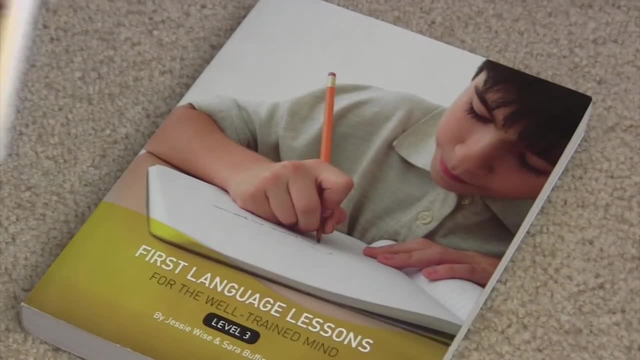 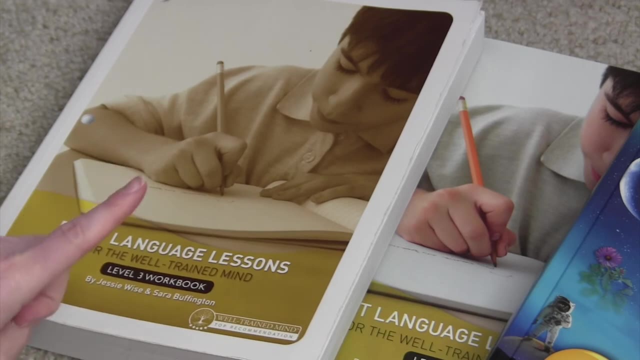 that is my review of first language lessons, level three from the well-trained mind. i will link the well-trained mind below and i will put the link in the description box below for you. so i hope you'll trained mine below and, of course, all of the other reviews that I've done, If you enjoyed this be. 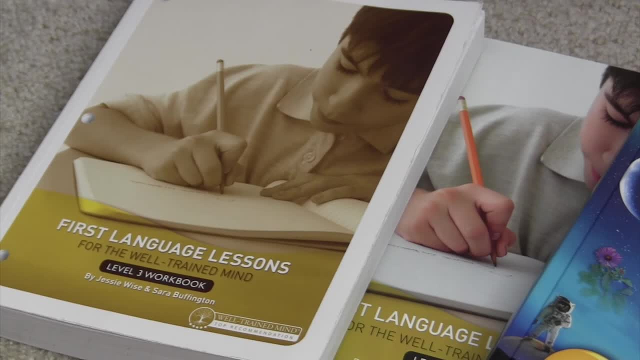 sure to give me a thumbs up. If you have any questions or comments or anything, please leave those in the description- I'm sorry- in the comment section below and I will do my best to get back with those. If you would like to see anything kind of along these lines, let me know as well. 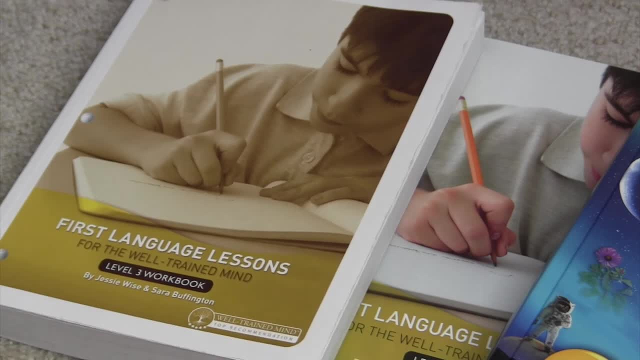 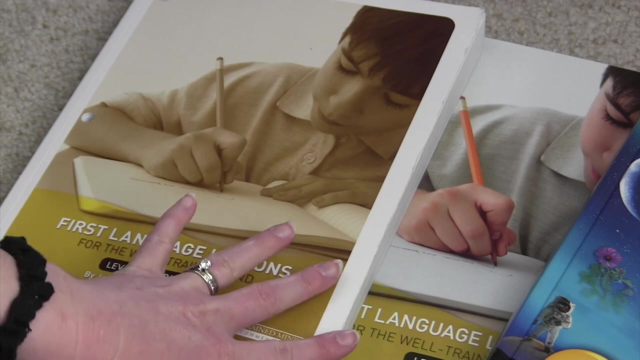 I love everything that I've ever bought from the well-trained mine. I kind of lean classical as far as education goes. It's just what works best for my mind. Does that mean it's for everybody? Absolutely not, but I think that this is a wonderful, wonderful curriculum If you need to. 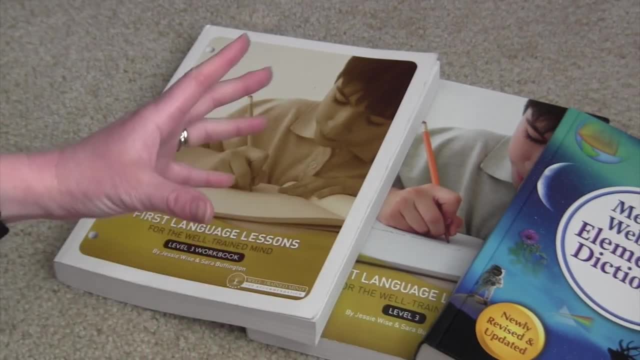 know kind of how to do this. if you're not sure how to teach grammar and writing and everything, this is a great place to start. Thanks so much for watching and have a wonderful day. Bye.